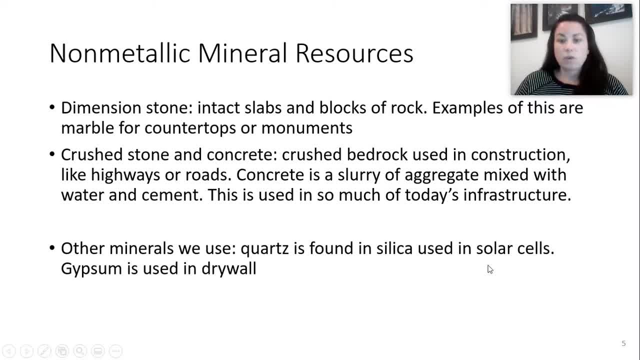 Some of the other materials or minerals that we use are things like quartz, which is found in silica, used in solar cells, or even gypsum, which is used in drywall. So we talked a little bit about this. We went over minerals a long time ago in class, But we have to think about where we get them and 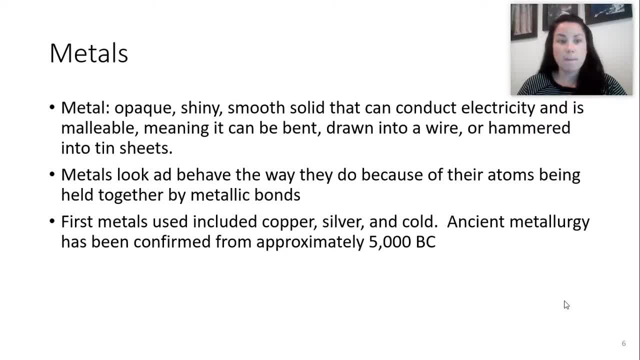 how we find them. Okay, so the other source is metals, and these are shiny, smooth, solid. that conducts electricity. It can be malleable, bent. we use it in wiring. we can be made into sheets and metals. look and behave the way they do because their atoms are being held together. 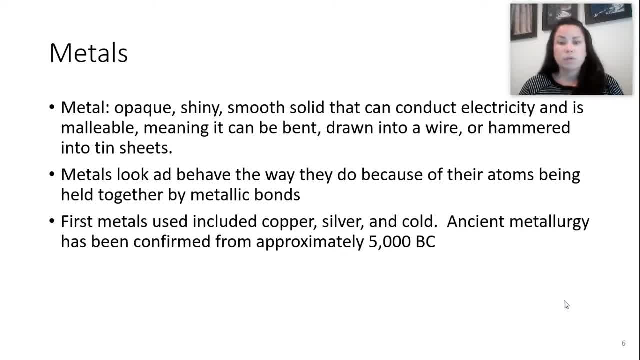 by metallic bonds. Some of the first metals we're using are in the form of glass and they're used to used to include copper, silver and gold. Ancient metallurgy has been confirmed from 5000 BCE, So metallurgy, the practice of melting and smelting and things like that, is quite an ancient practice. 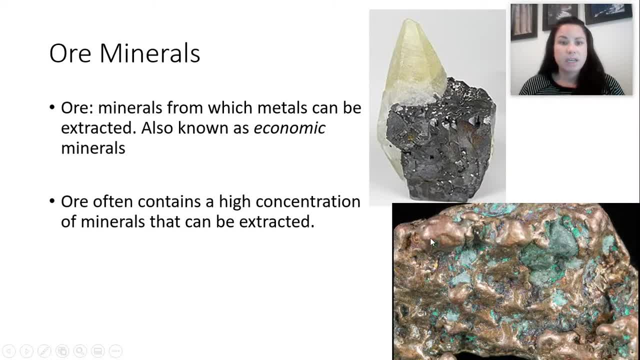 So here's an example of an ore mineral. This is minerals are which metals can be extracted, So like an economic mineral. so not every mineral is considered economic, And ore often contains a high concentration of mineral that that can be extracted. So here we have some copper. 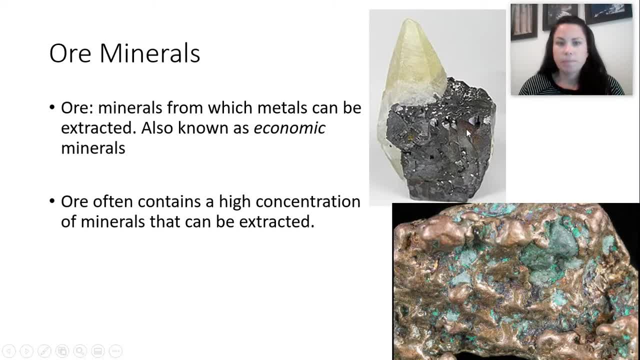 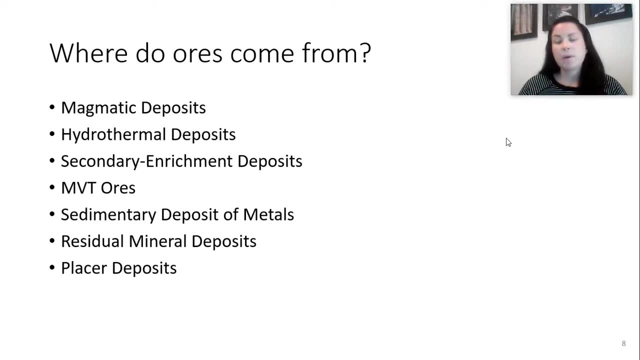 Up here this looks more like some pyrite or something. But whatever this is, it's a. it's a large quantity of a high concentration of that of that metal. So where does it come from? We're going to talk about each of these individually here. 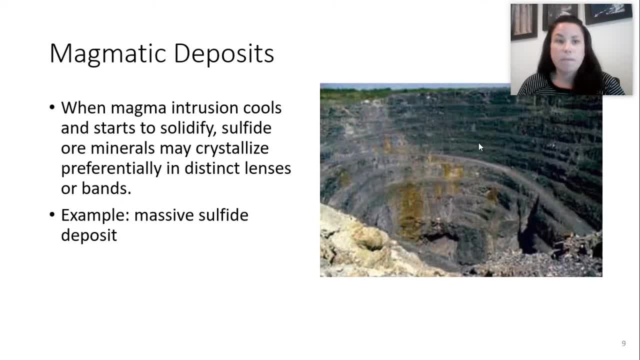 So the first is a magmatic deposit. This is when magma intrusion, when magma intrusion cools and it starts to solidify The sulfide ore, minerals may crystallize in distinct lenses or bands. An example of this is sulfide deposit. you can see in this picture here on the right. 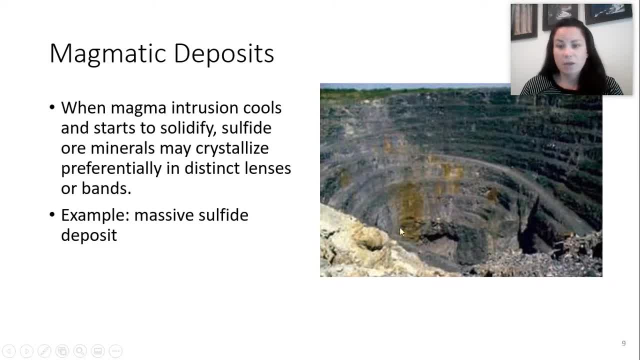 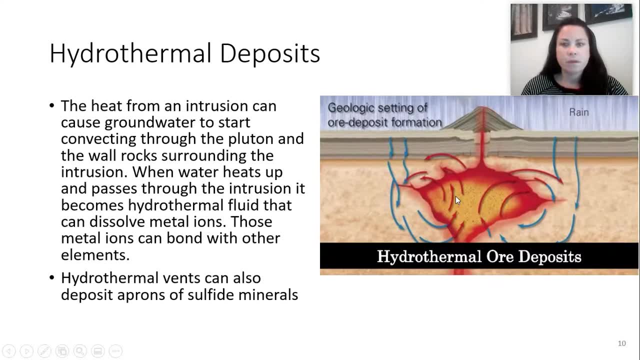 that this is an open pit mine And you can see the sulfide bands and lenses here. it's in that orangish color. We have hydrothermal deposits. This is heat from an intrusion can cause groundwater to start convecting through a pluton or a dike and the wall rocks surrounding the intrusion. 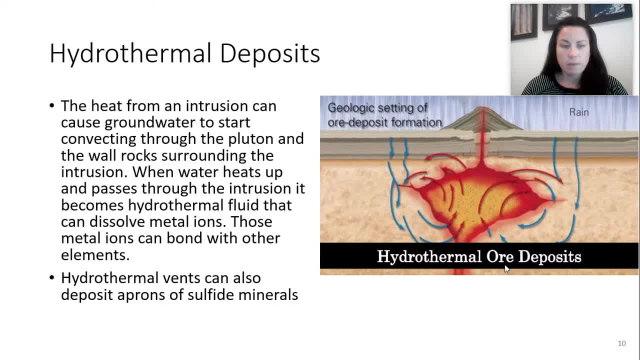 And when the water heats up and passes through it, it becomes a hydrothermal fluid that can dissolve these metal ions, And then those are carried with the fluids and they can be deposited in these hydrothermal vents through near a volcano or through. in this case, we have rain that is coming down and cooling the magma around an intrusion and 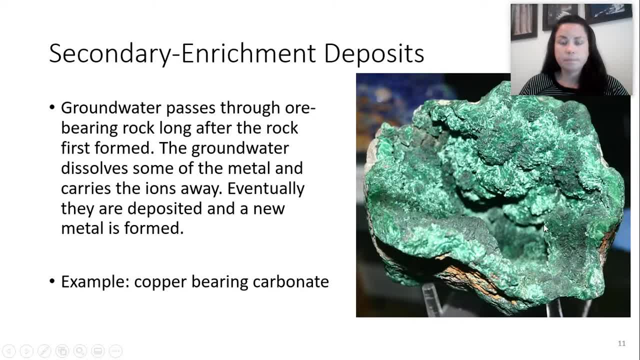 creating these hydrothermal deposits. Okay, next is a secondary enrichment deposit. This is where groundwater passes through ore-bearing rock long after the rock has first formed, And then the groundwater dissolves away some of the metal and carries those ions with it, And then eventually, as the water carries these ions, they can be deposited and a new metal is. 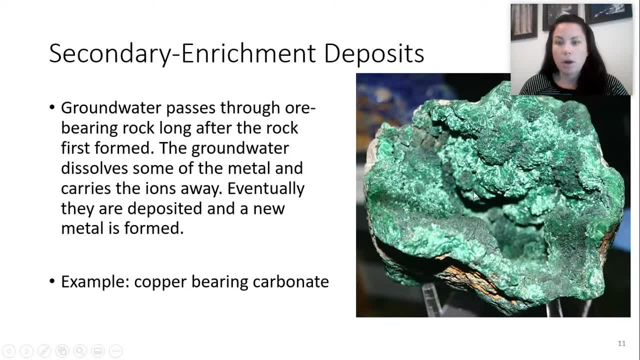 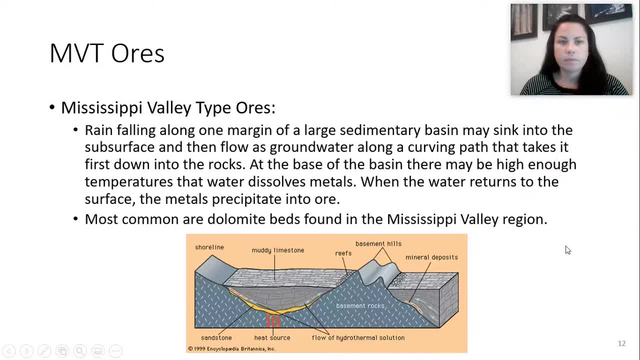 formed. So an example of that is a copper-bearing carbonate. So this is an example of copper here in this greenish color. Okay, next is a Mississippi Valley type ore. This is a really specific type and this is a really common type of ore that we have in Mississippi Valley. So what happens is we have rain. 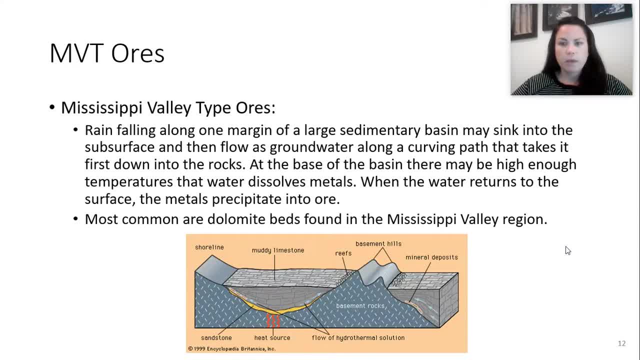 falling along one margin of a large basin and it sinks into the subsurface And then flow- groundwater flow takes it down into the rocks And that the base of this basin is where we have a heat source, or, if there's enough pressure below it, they can dissolve these metals. 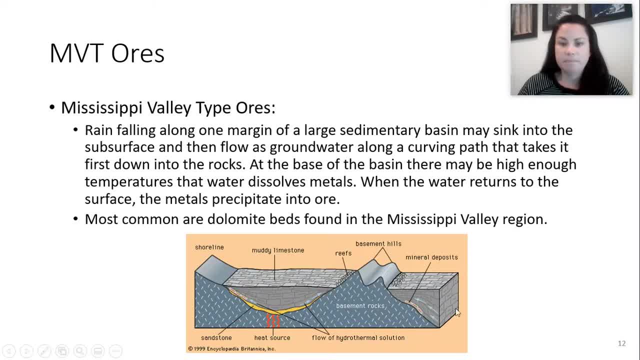 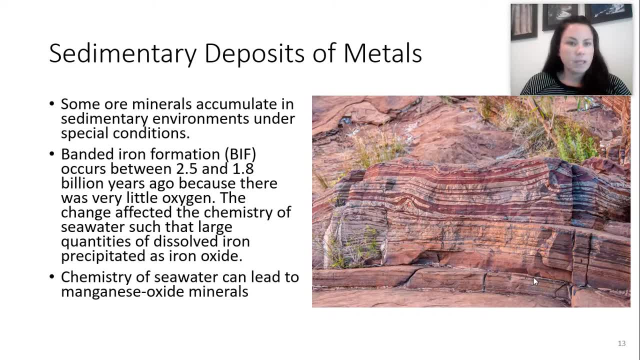 And this is a specific type: Valley region. Okay, sedimentary deposits of metals. Some ore minerals accumulate in sedimentary environments under some of these specific conditions, where we have- here's an example of banded iron formation which occurs between 2.5 and 1.8 billion years ago, because there is 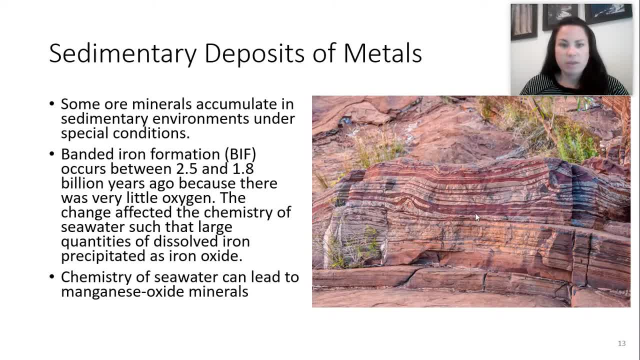 very little oxygen. So this is a regional trend that we see The change effect of the chemistry of seawater such that large quantities of dissolved iron precipitated as iron oxide And the chemistry of the seawater can lead to manganese oxide minerals. So these banded iron 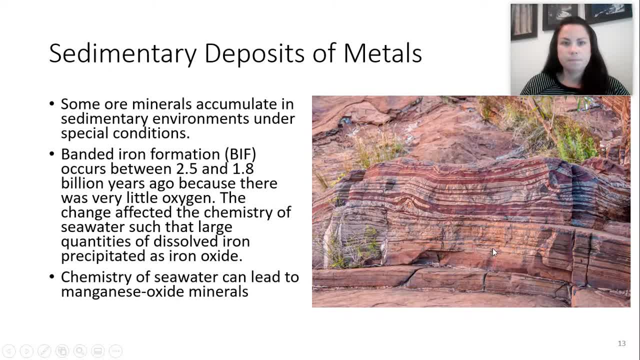 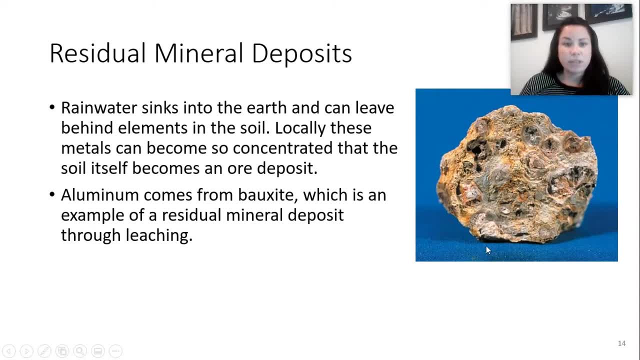 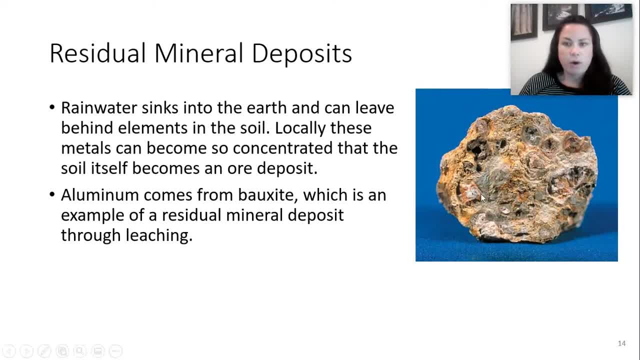 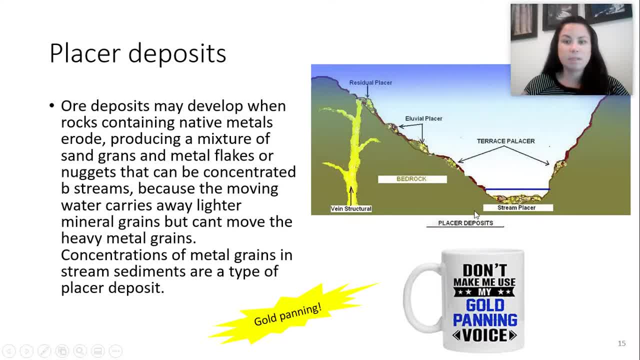 okay, next is placer deposits. these are ore deposit, and this is generally when we think about mining. most of the mining that we think about in terms of metals come from placer deposits. this is where ore deposits may develop. when rocks containing native metals erode, they produce a 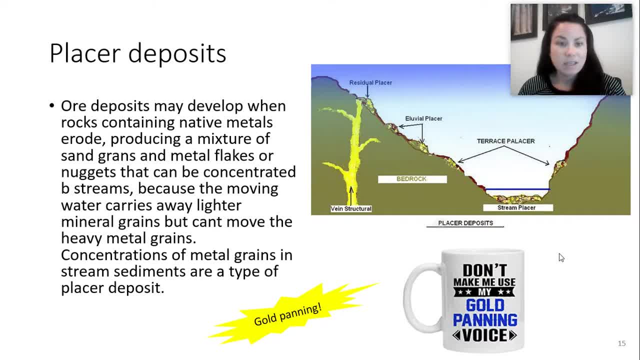 mixture of sand grains and metal flakes or nuggets that can be concentrated by streams, because the moving water carries away lighter minerals but can't move the heavy metals. so concentrations of metal grains in stream sediments are a type of placer deposit, and this is where we 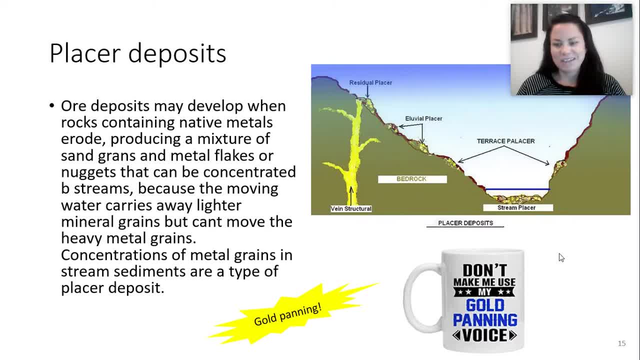 might see. if you've ever watched anything on on whatever tlc about gold panning or gold digging and things like that, you would. you'd be interested in placer deposits because running water can can carry some of these heavy metals. um, if you've ever done gold panning, it's a lot of fun. i forgot. 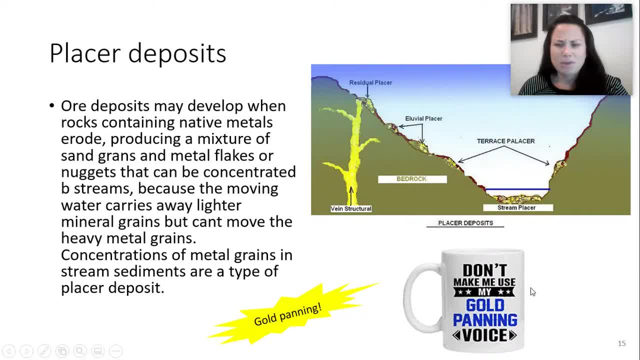 that i put this picture in here. um, that's hilarious. so don't make me use my gold panning voice. i don't even know what that means, but if you've ever done gold panning, it's a pretty fun exercise because it's it's quite relaxing. it's maybe akin to, um, you know, doing a puzzle or 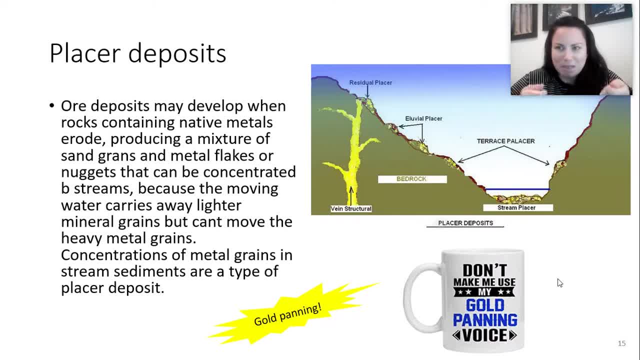 something: you're there with your little gold pan with your sediments and you dip it in water and you shake it out and you allow the sediments to um settle and the heavier metals settle out at the bottom of your pan. you can collect those and melt it and and um say that you've found gold. you know, going down the 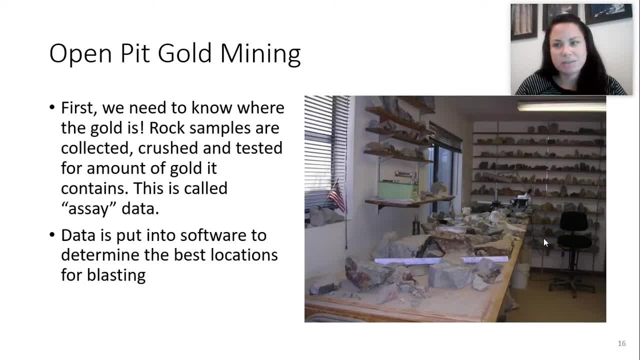 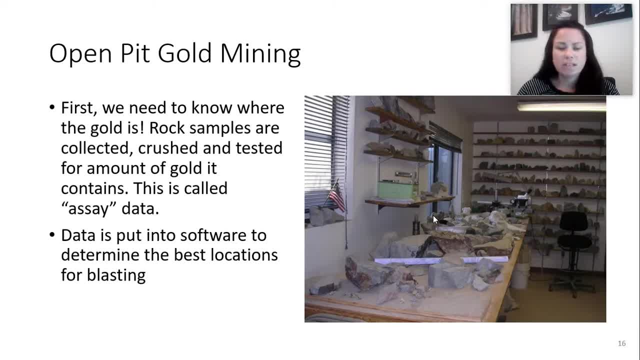 so we would look through some of these rock samples that were collected. we'd crush them up, do a test on them to see what the concentration of gold was on these rock samples, and then we would use modeling software to say: you know, x marks the spot of where. 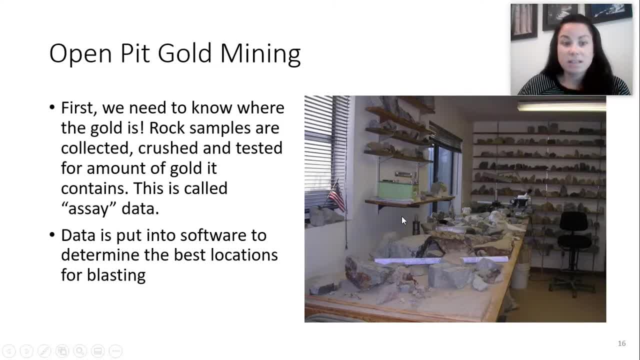 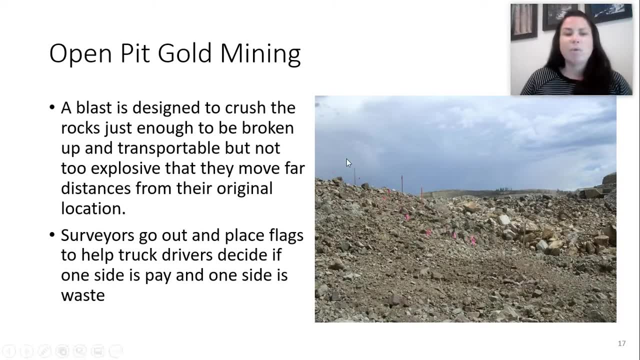 the highest concentration of gold was based on these assay data. and then, in this open pit gold mine, what we would do is we would blast the rocks so we would create zones, um of fractured rock. basically that would be moved and sent to either the disposal pile or sent to the crusher. and so, um, again, doing that assay data. 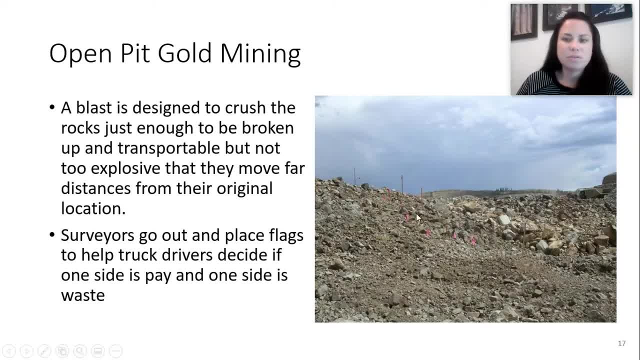 said basically, like you know, x marks the spot. or what we would do is use survey flags to say: dig anything over on that side, um, and send it to the crusher. or dig anything on that side and send it to the disposal, because we want to keep, uh, the, the rocks that had the most gold in it. 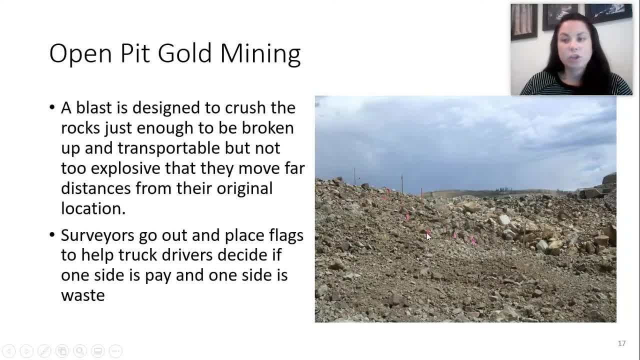 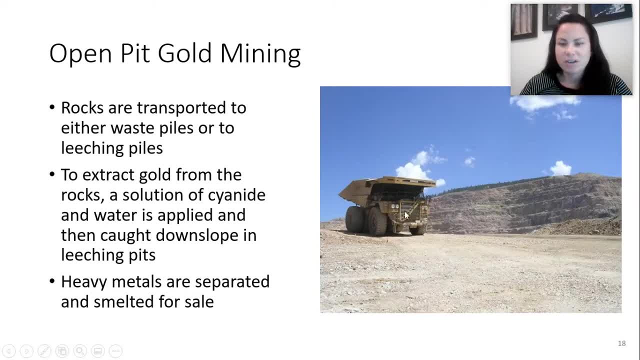 um, so these indicators were used for the, the large trucks that would come in and plow these rocks. so here's- here's a picture of one of those trucks. it's hard to see the scale on here, but if you can imagine that there's a guy sitting in here and driving 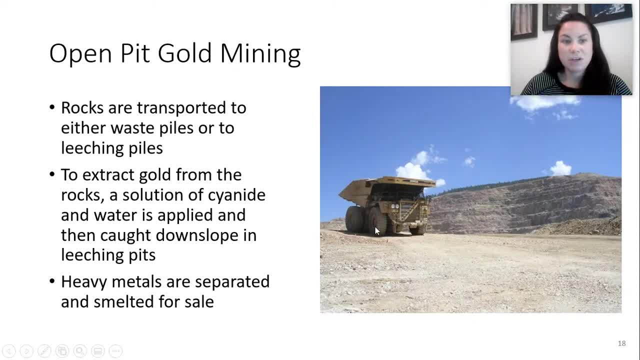 these tires are probably at least 10 feet tall, so there's quite a large truck. so these rocks would be then transported to waste piles or leaching piles, and to extract gold from the rocks they would have to pour a solution of cyanide and water in order to basically leach the metal out of the rocks. 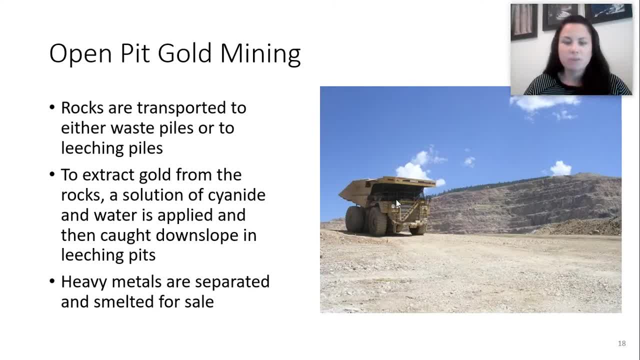 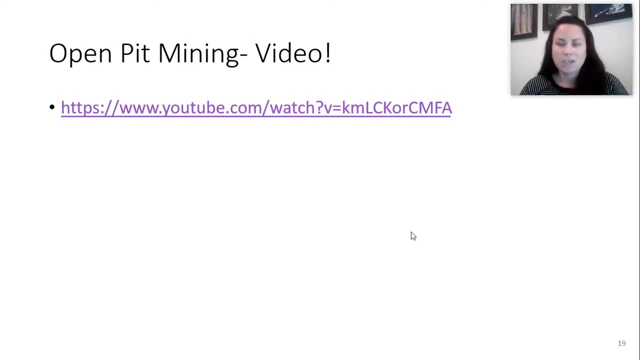 and they would be collected in ponds along with all the chemicals and they would be separated and melted and sold and all of that. but this is a quick glimpse of um of what the uh, the procedure was for looking for the gold, for gold, in an open pit gold mine. 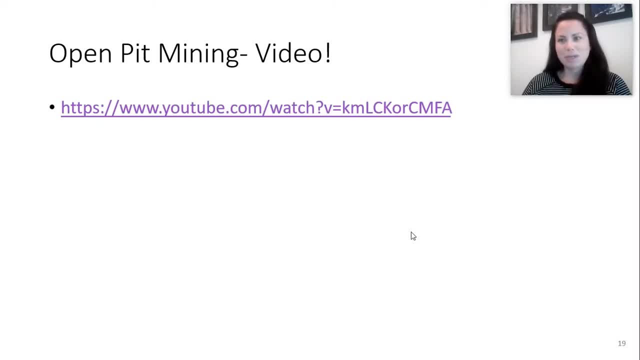 And where I worked is actually they have their own promotional video. So here's a quick run through of some of the facilities of the gold mine in Cripple Creek, Colorado. So check this out: 177 M3 ready and standing by. 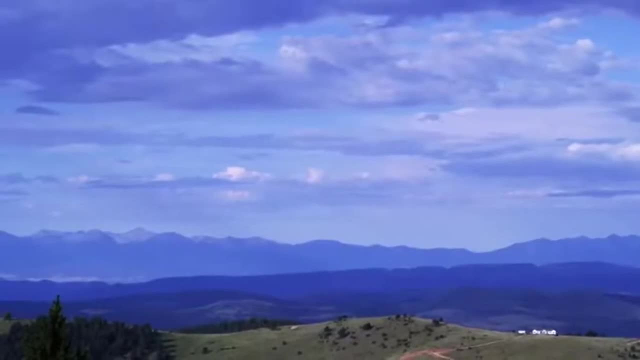 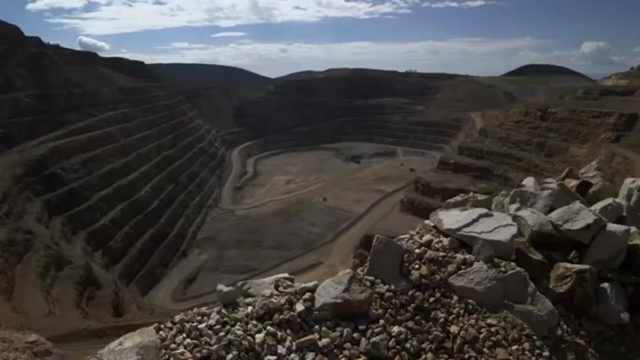 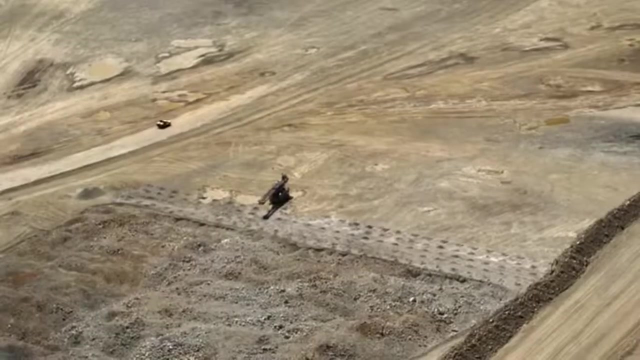 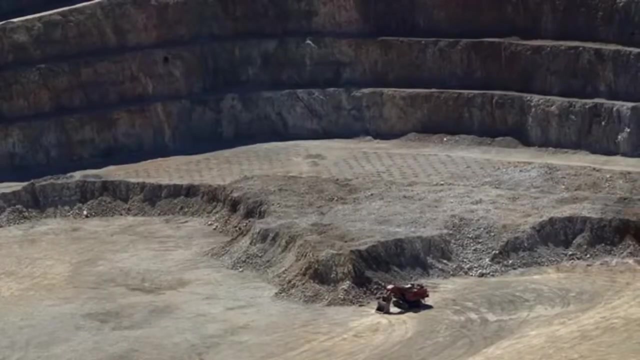 This is your final warnings for shots going down the pit on the 9445.. We'll have the blast iron at this time, All units. we'll have a five second countdown before detonation. Five, four, three, two, one. 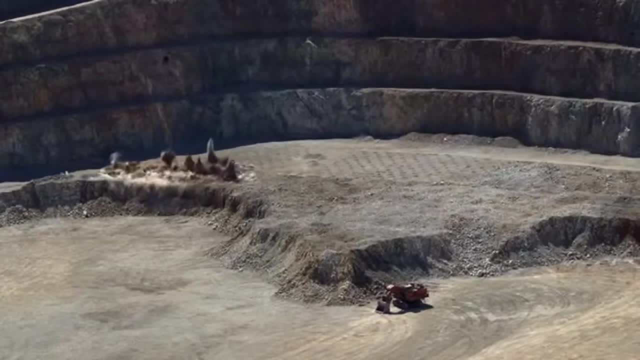 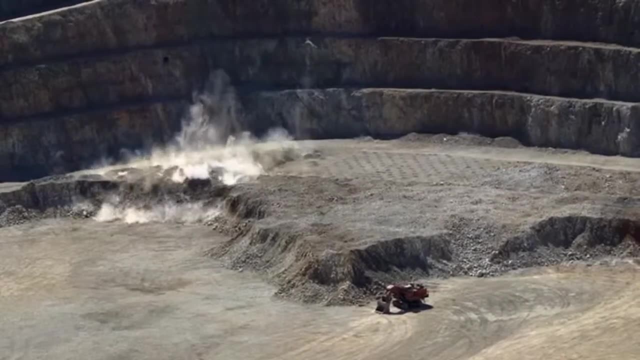 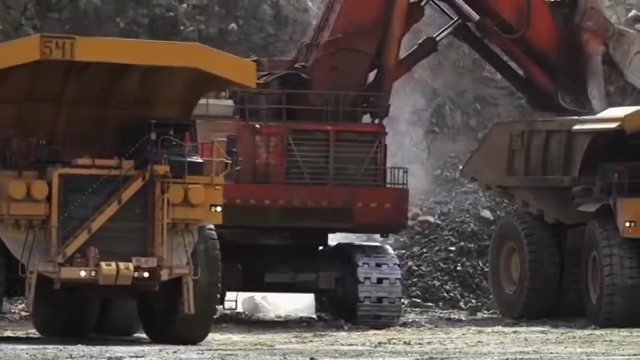 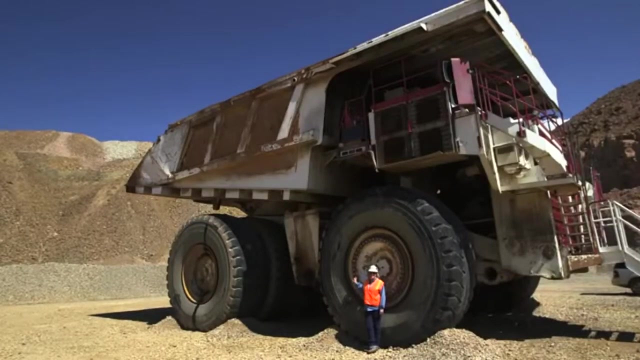 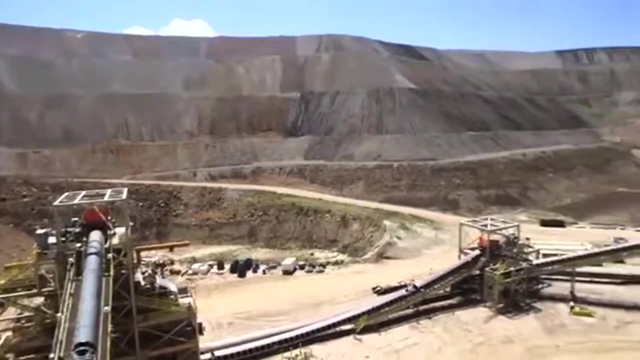 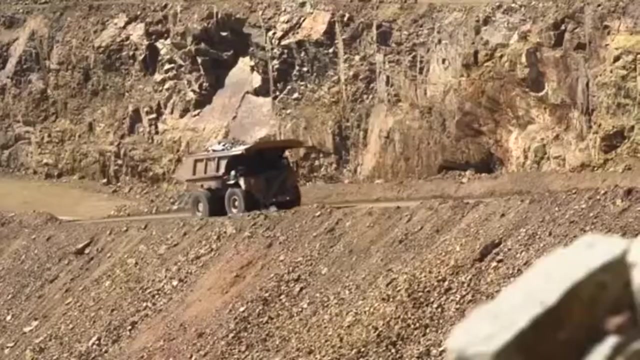 Fire in the hole. My name is Jane Manon. I am the manager of community affairs for the Cripple Creek and Victor Gold Mining Company. The ore that goes to the crusher: we crush that to about a three quarter inch size. We convey that up to a load out bin that loads trucks. 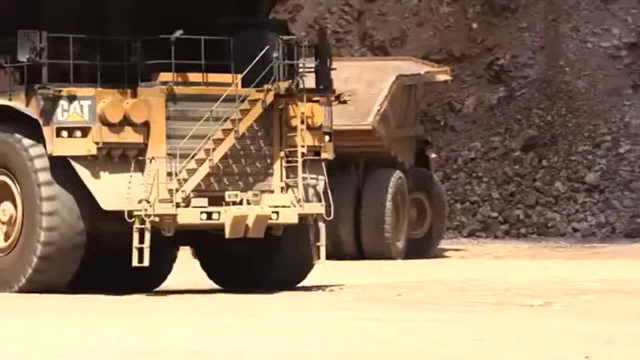 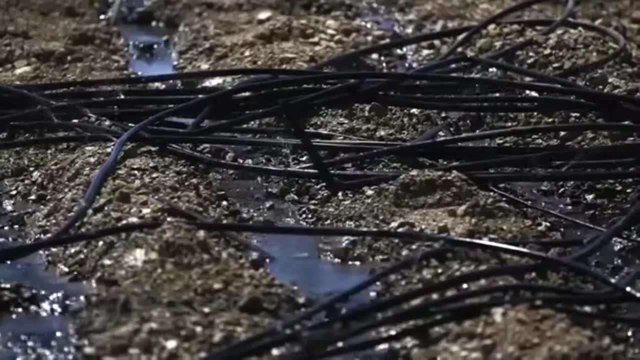 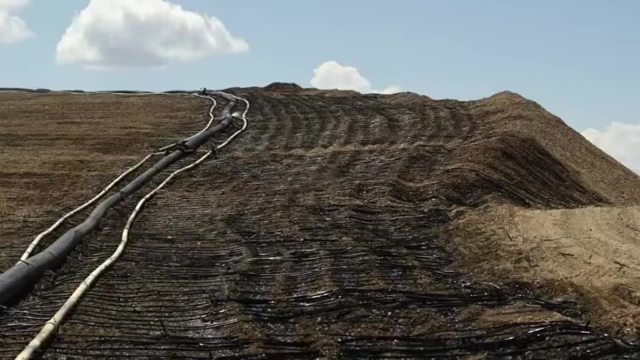 takes it out onto our valley leach facility. We stack the ore on top of that kind of like putting rocks into a bowl. We sprinkle a dilute sodium cyanide solution on the top of that ore. It dissolves the gold and we also get a little bit of silver. 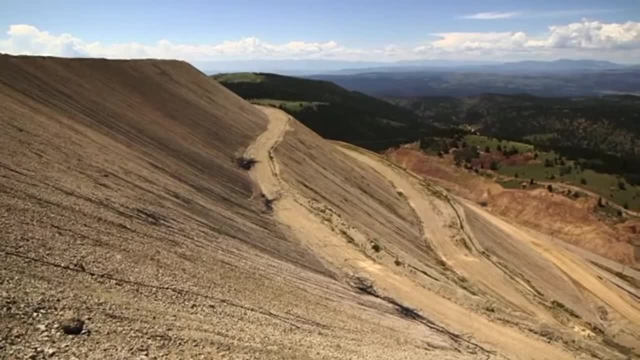 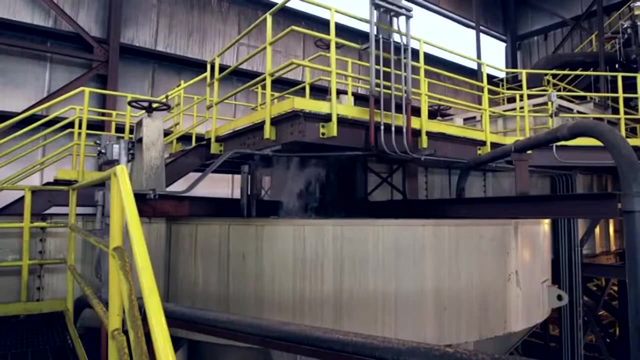 that's on the surface of the rock And it sinks down to the bottom of the lined area. We pump the solution out of the bowl into our processing plant, where the gold is filtered out through a series of carbon columns When that solution comes in. 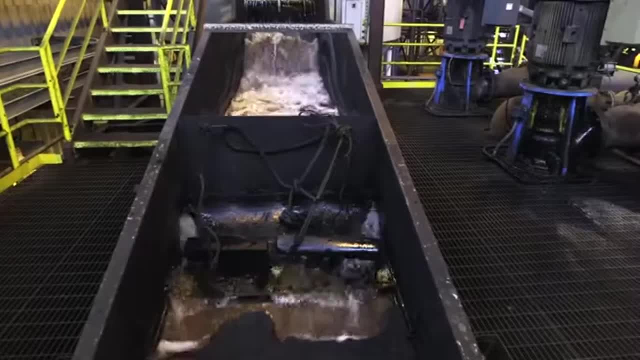 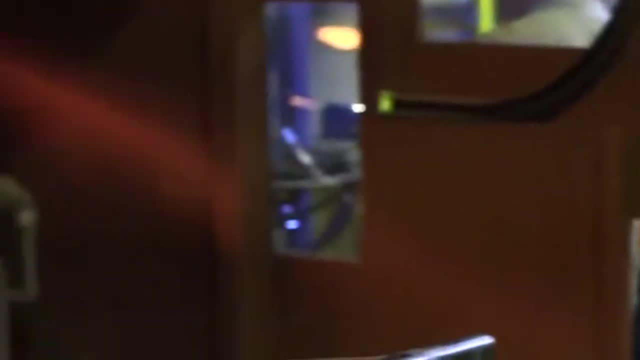 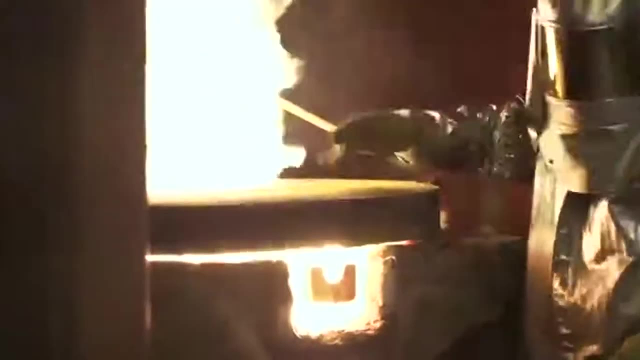 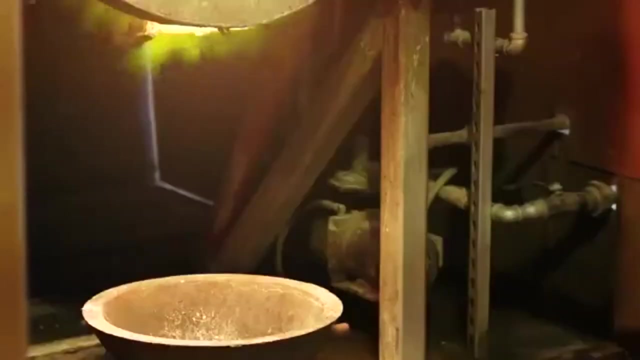 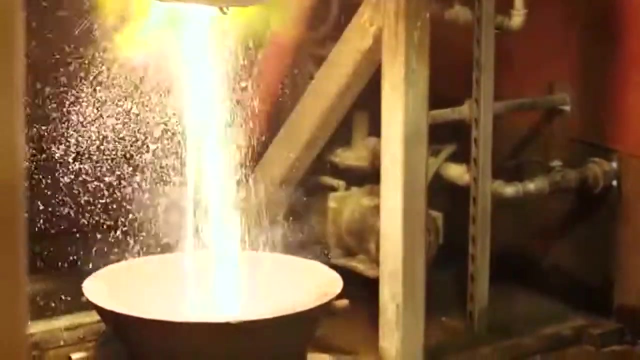 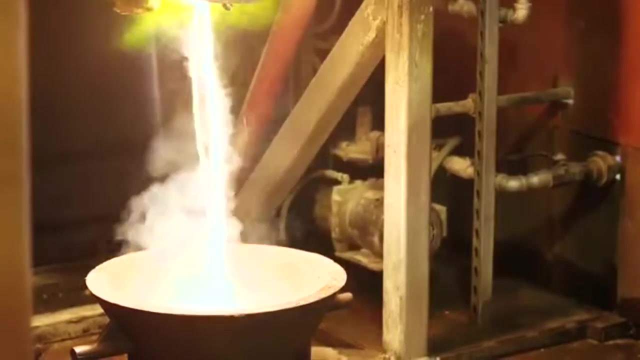 to the plant it looks just like water. You really can't see the gold in it at all. We strip the gold off the carbon, put that into the refinery with some silica and some other flux agents. The gold and silver are heavier. 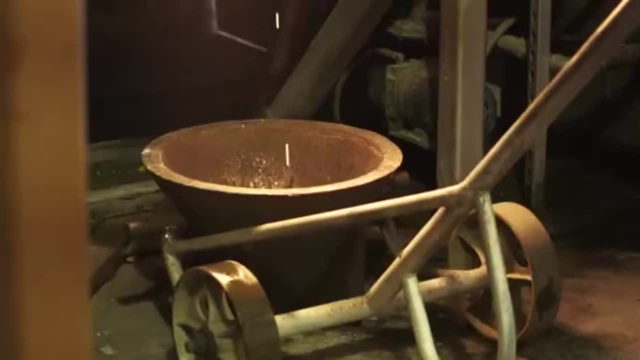 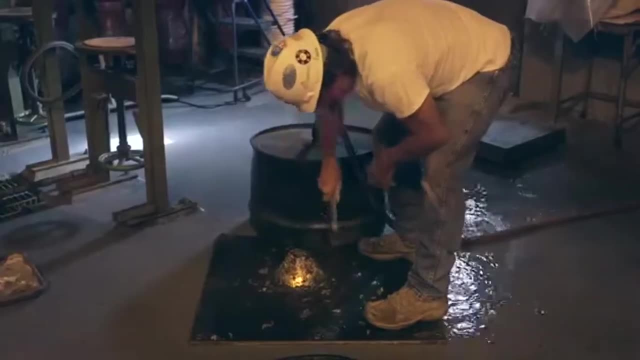 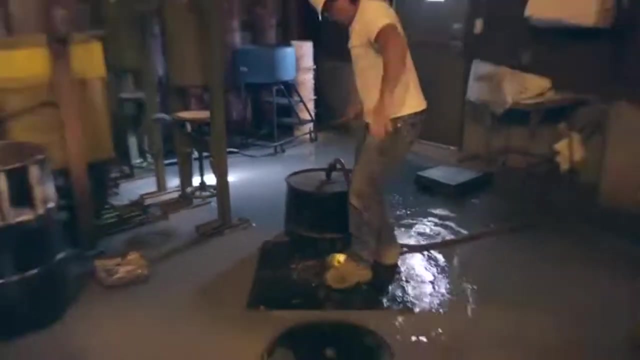 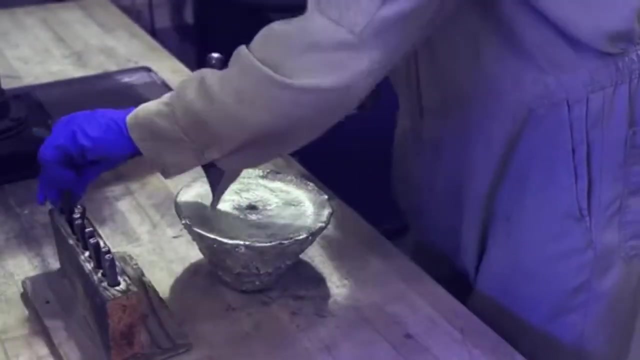 They sink down to the bottom and that silica forms a layer of almost like a glass type material on the top. We want to have it. so there's nothing that isn't gold and silver. so when we weigh it we can say to the refinery: this is how much it weighs, this is gold and silver. 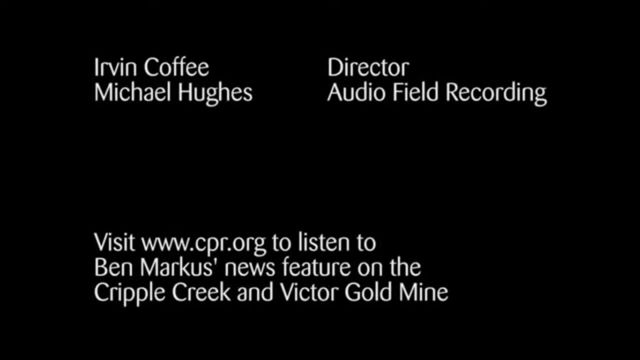 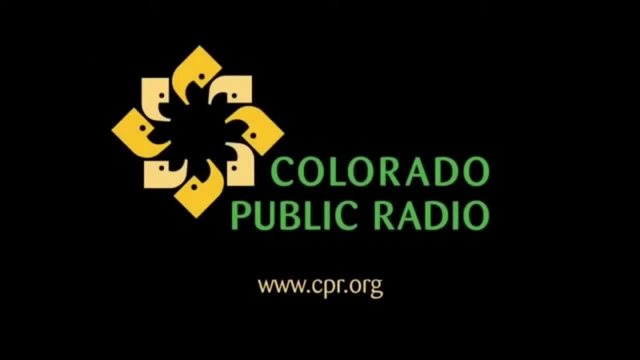 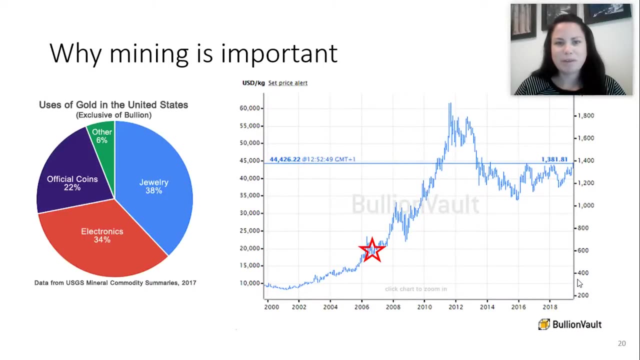 Every time I watch that video of the Crypto Creed gold mine, it makes me reflect back on how crazy I was as a 19-year-old as an intern working in a place like that. It's very interesting, geologically interesting, to think about. 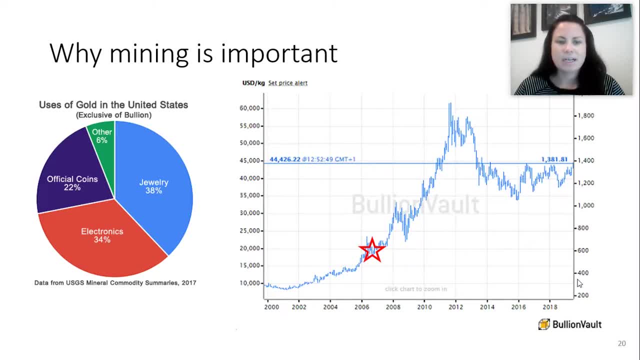 How gold and silver work, Gold deposited there, where the gold deposits are, and all that stuff. It's very interesting, but I also have to remind myself of how crazy it was to work in such an interesting environment. Why is mining important? This chart is a little bit dated, but here's specifically for gold. 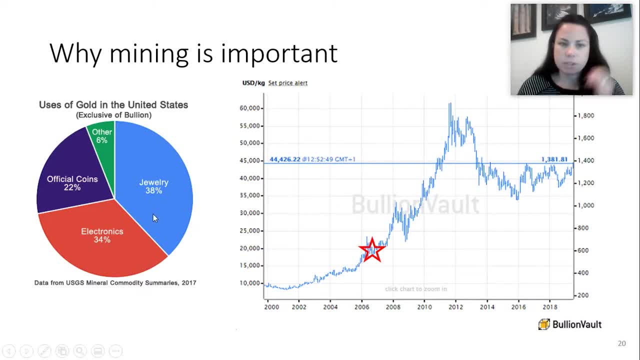 Uses of gold in the United States is broken up here on the left and this is from 2017.. But a lot of it is from jewelry and I imagine, now that electronics have exceeded that metric, that we use more gold for electronics. I guess gold is also used in coins and a few other things here. 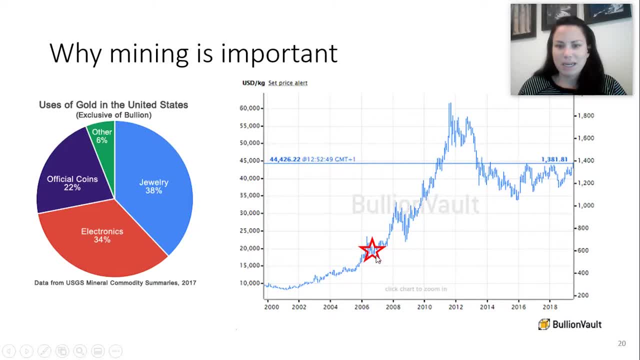 Now, when I was interning at the gold mine here in 2006,, this is the price of gold around $600.. I really wish I invested some money then, because this chart goes until 2019.. Roughly, where gold was around $1,400, now today it's around $1,800, so it's really come. 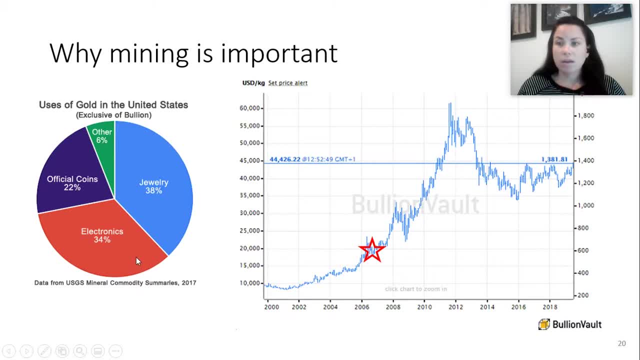 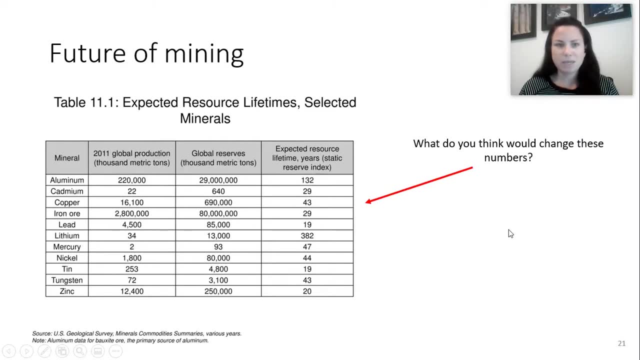 back up in price, and I think that's because we are relying on precious metals like gold for electronics. So let's talk about the future of mining. What does that look like? Well, here's a chart of the expected resource lifetime for selected minerals. here: 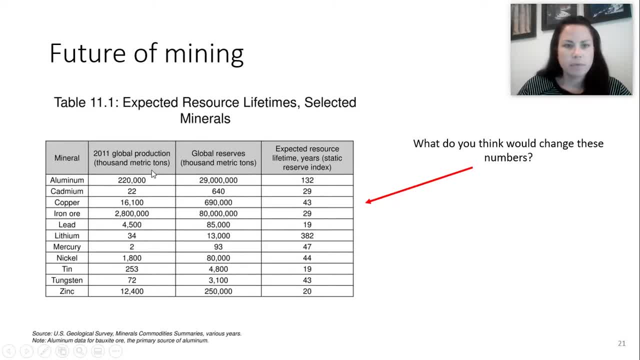 So we see that in 2011,, this is how much has been produced. This is how much is in reserve and the lifetime of those reserves, based on our current consumption. So let's look at. we should be okay with aluminum. we have 132 years left of aluminum. 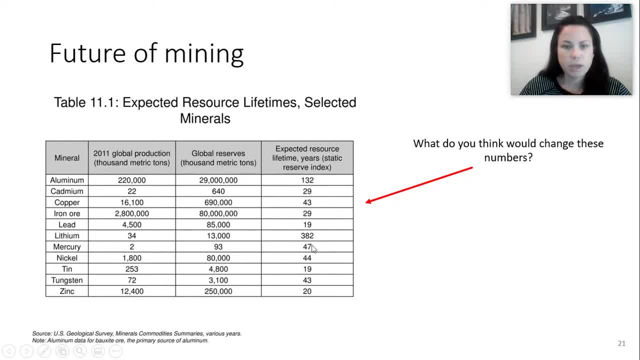 But some of these other numbers, like look at lead, that's quite low. tin is also low. So when we look at these numbers and what that might mean, what do you think would impact those numbers? How do you think we could change the life of an expected resource? 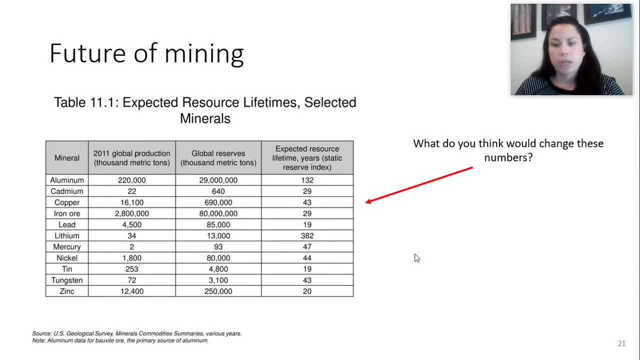 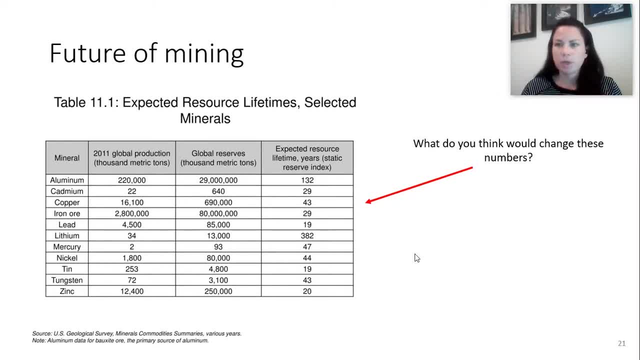 Yeah, Yeah, Yeah, Yeah, Yeah Yeah. Just something to think about as we consume and consume, and consume. when we have electronics and we keep building and we keep having more stuff, It's not forever. A lot of these processes that I just showed you, with deposits, those take millions of years. 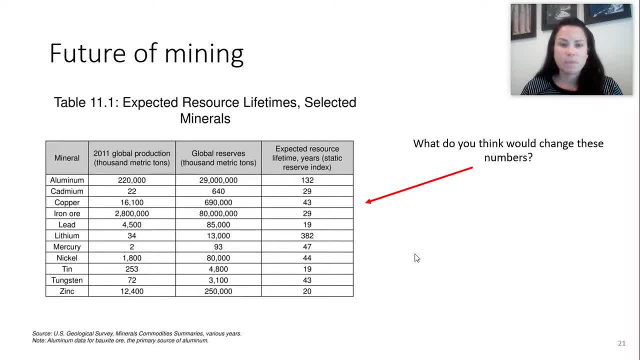 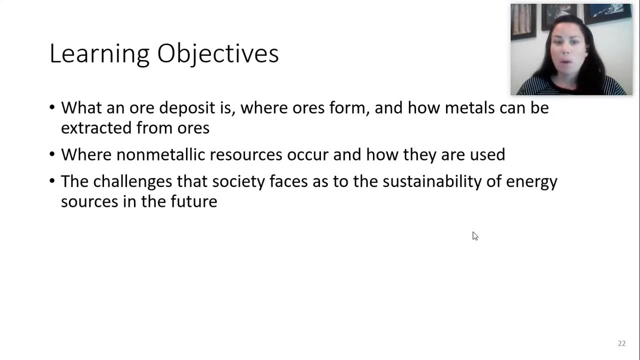 to occur and we're stumbling upon it and finding a use for them, So it's not like it's a renewable resource in any way. So we have to think about our consumption and how sustainable that is for some of these resources. Okay, So, in brief, we talked a little bit more about metals in terms of mining, but we talk about 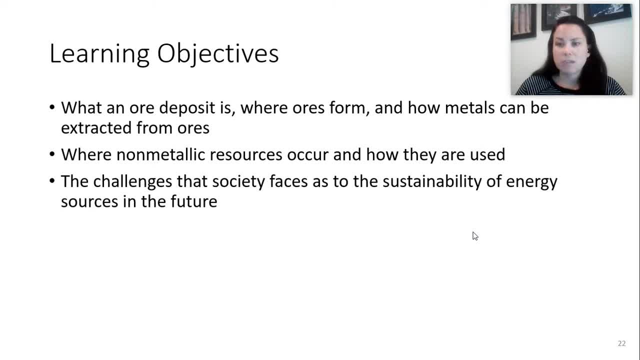 the non-metallic resources. in the context of minerals, I had a video on granite and creating sculptures out of them and things like that. So we use a lot of other resources and mining as a way that we can extract those resources And, of course, we have some challenges about sustainability. 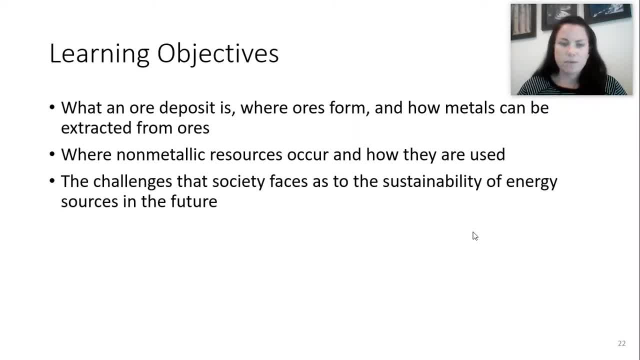 And our use of these resources in the future. See you next time.